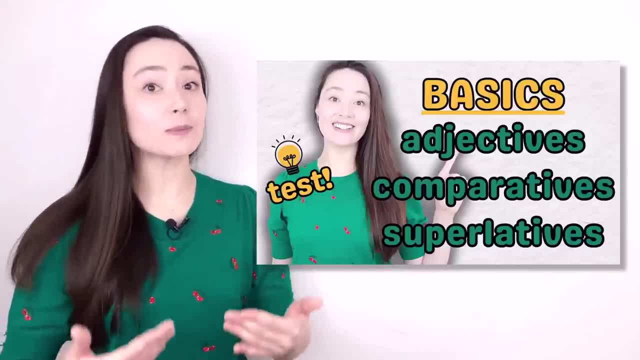 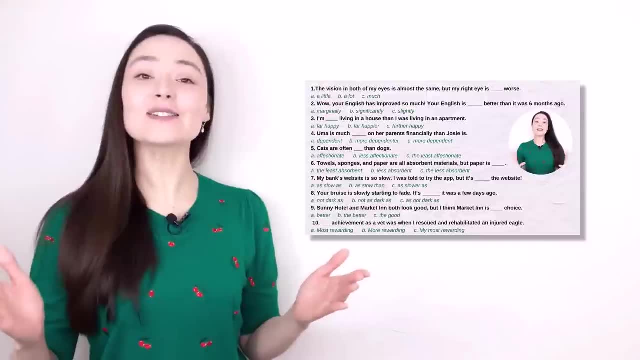 the basics of adjectives, comparatives and superlatives, which I'm not going to go over in this lesson. At the end of this lesson, I have a test for you with 10 questions. Please let me know if you have any questions. If you have any questions, please let me know in the comments. 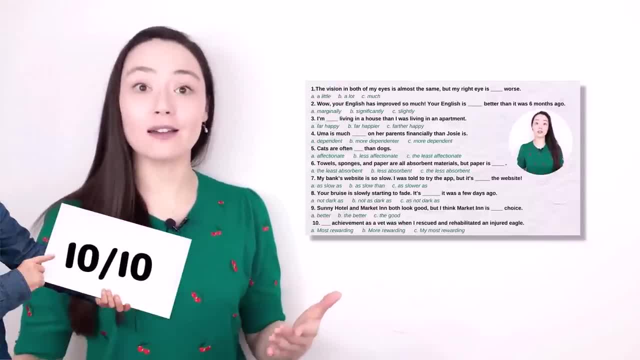 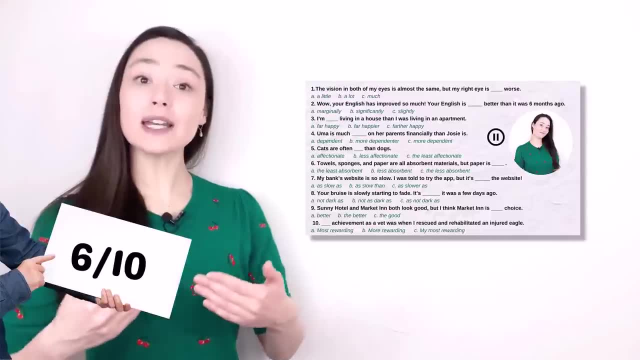 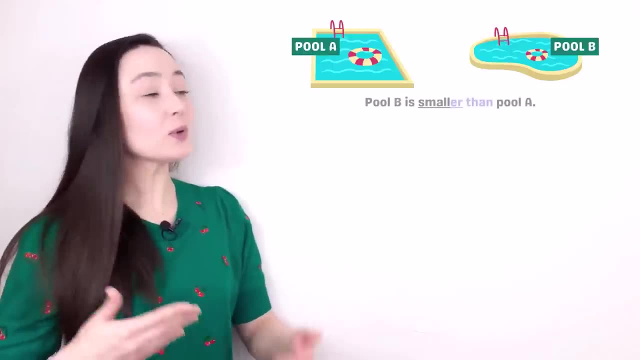 Let me know your score in the comments below. Did you get 10 correct out of 10?? Maybe 6 correct out of 10.. Let me know My name's, Arnel. Let's start. I have two pools. Pool B is smaller than. 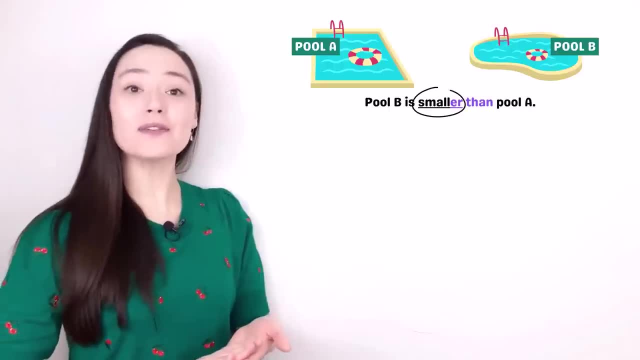 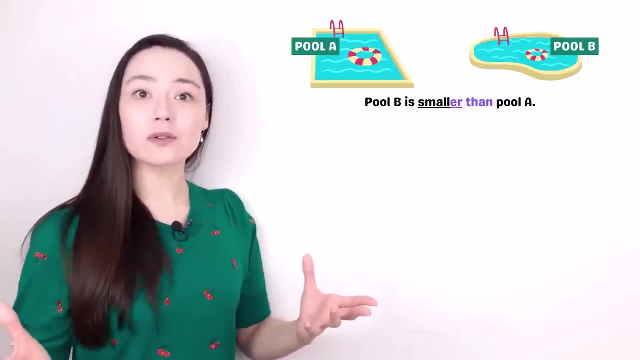 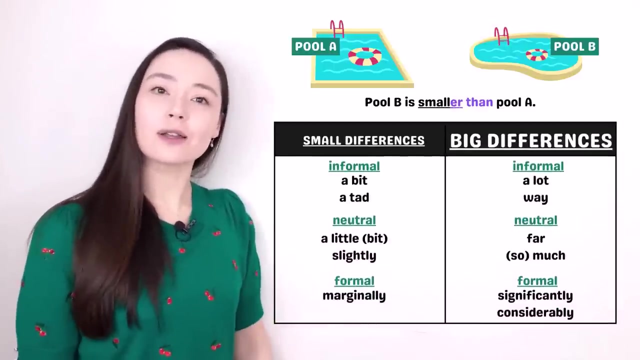 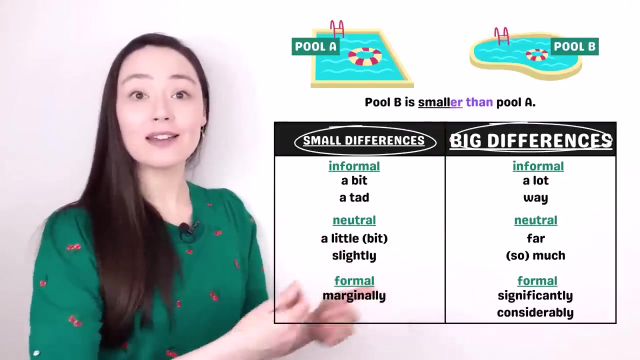 pool A, I have my comparative and than because I'm comparing two things. This is correct, but it's very general. How can I be more specific? I think we need a chart. Maybe you haven't noticed, but I love charts: Small differences, big differences. Informal means we normally use these modifiers. 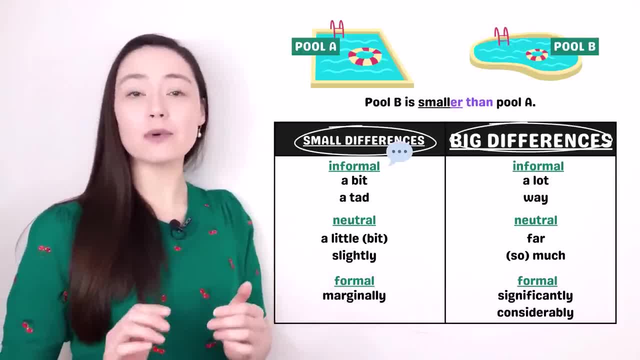 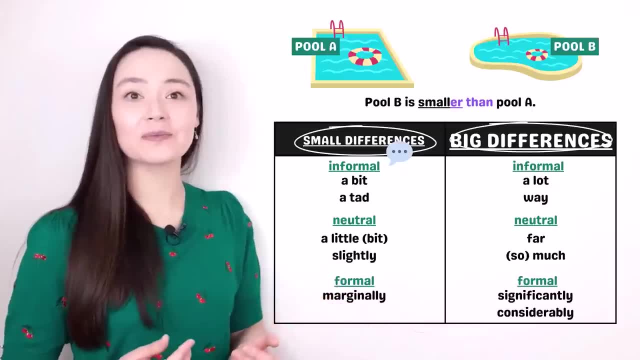 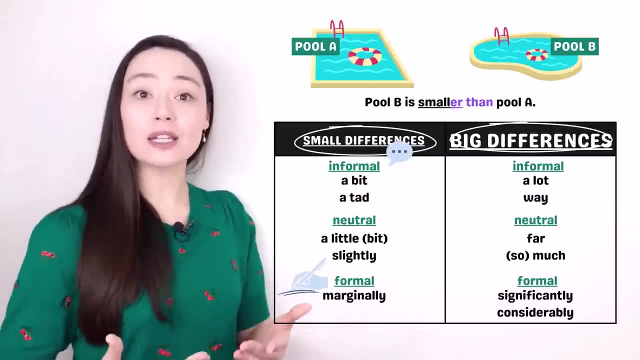 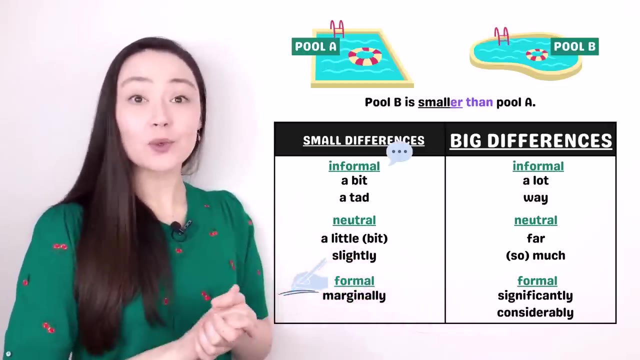 in spoken English And it's important to remember informal English does not mean low level English. Informal English is very natural. Then neutral and formal Formal meaning you'll normally see it in written English And this chart is just a guideline. These aren't strict rules. Pool B is smaller than pool A. 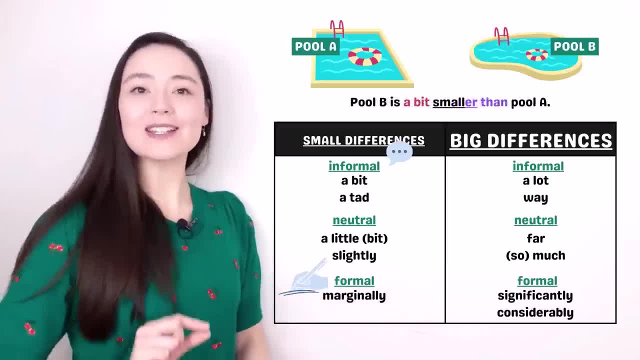 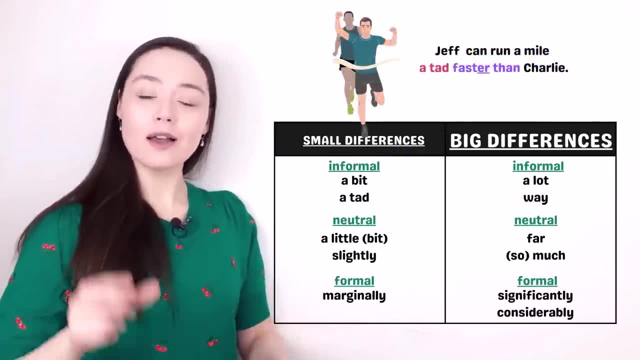 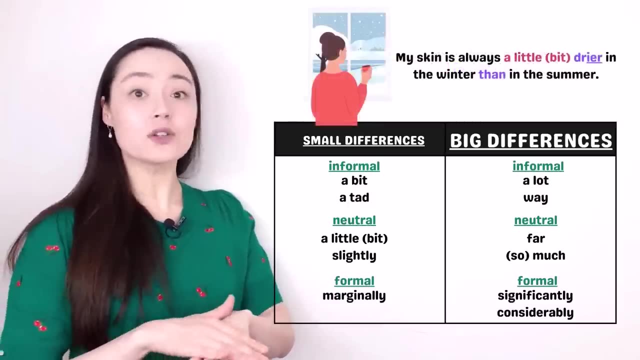 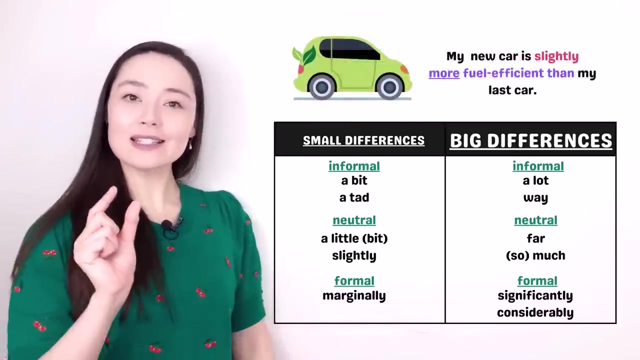 Let's be more specific. Pool B is a bit smaller than pool A. Small difference. Jeff can run a mile a tad faster than Charlie. My skin is always a little drier in the winter than in the summer. My new car is slightly more fuel efficient than my last car. 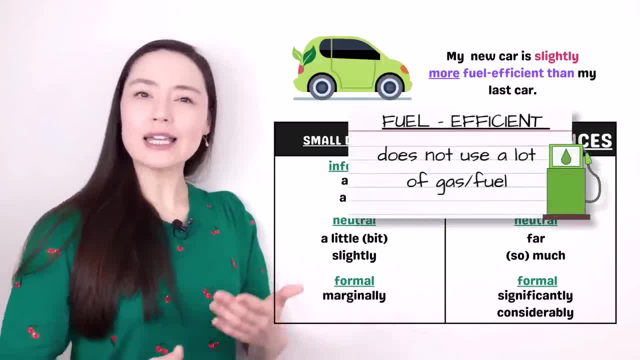 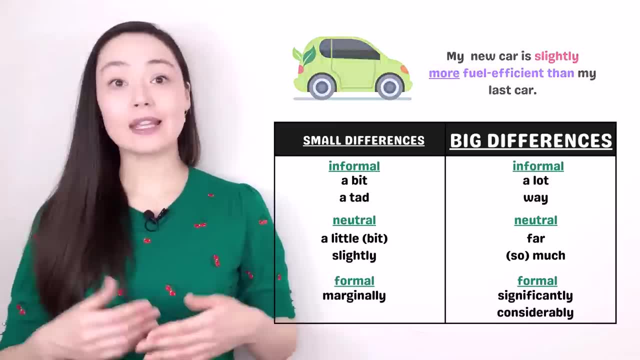 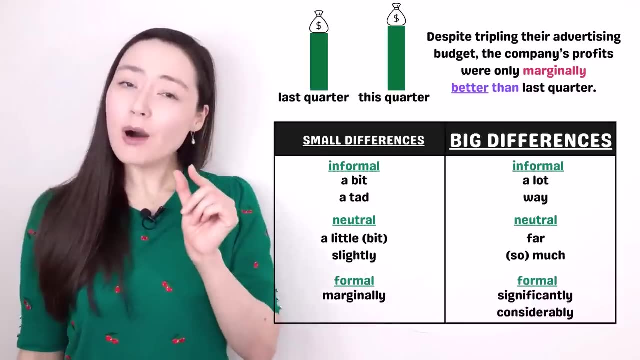 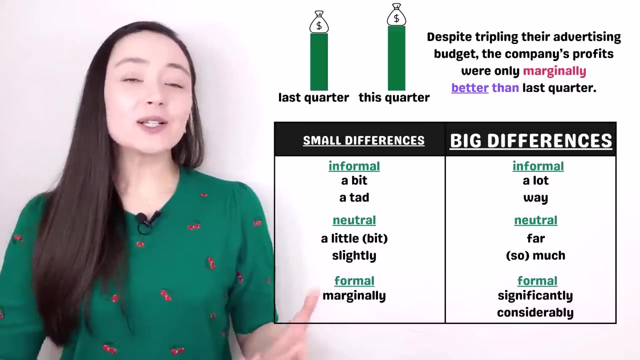 Fuel efficient means it doesn't use a lot of fuel. It doesn't use a lot of gas. Small cars are normally more fuel efficient. Despite tripling their advertising budget, the company's profits were only marginally better than last quarter, And you don't need to include van plus the object if 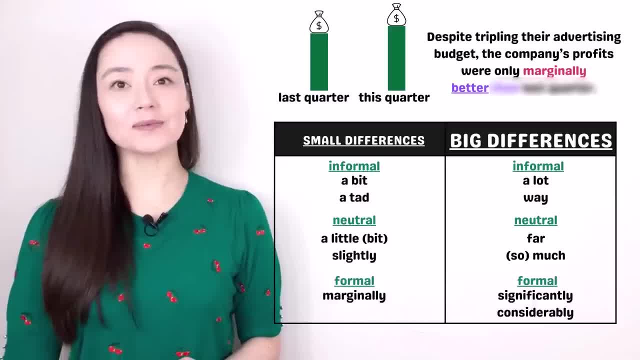 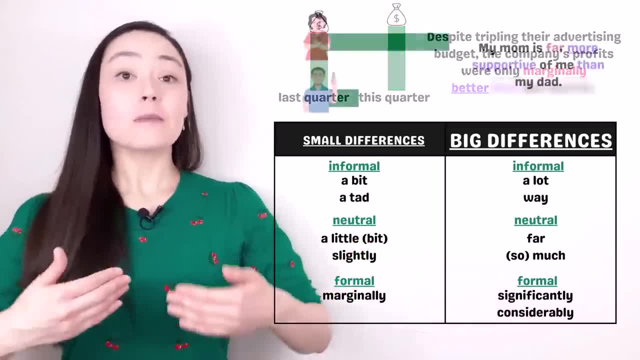 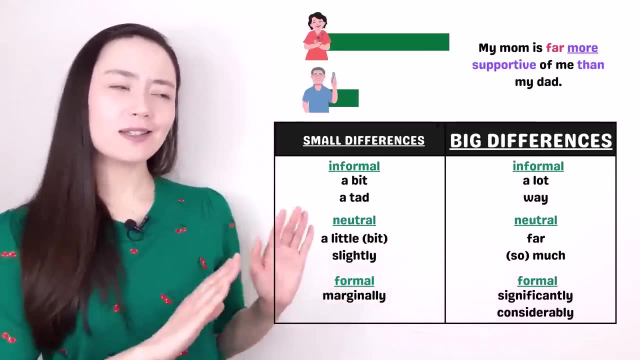 it's already clear what you're talking about. That's optional. We've looked at small differences. Let's do some big differences. My mom is far more supportive of me than my dad. This is just an example. In my life, my parents are equally supportive. 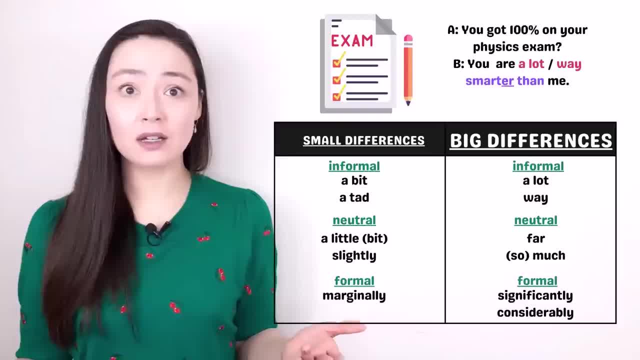 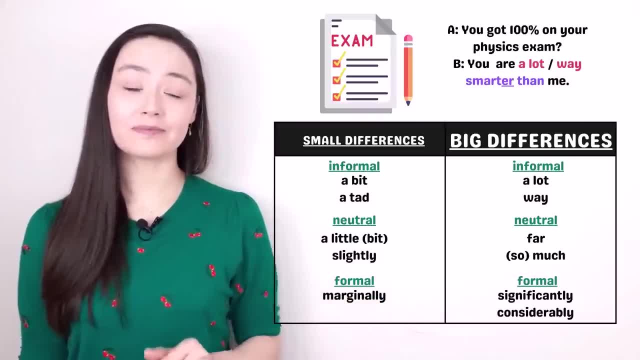 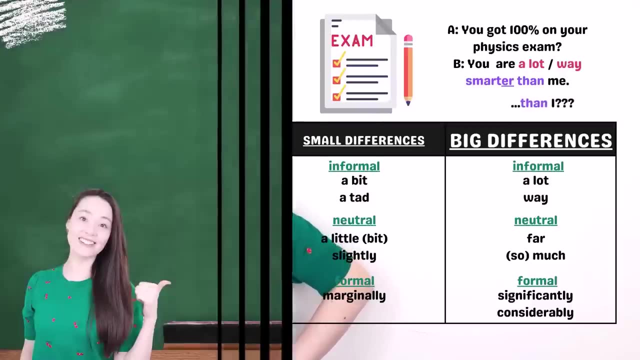 You got 100% on your physics exam. Wow, you are a lot smarter than me. You are way smarter than me. Smarter than me? or smarter than me? Smarter than I? Okay, we need to get into the nitty-gritty of the grammar. 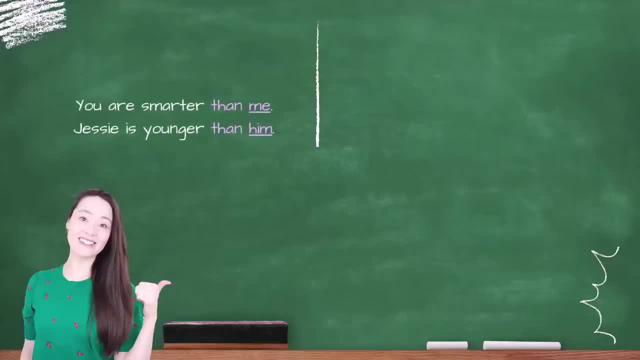 You are smarter than me. Jesse is younger than him. You are smarter than I: Jesse is younger than he. Which side is correct? They are both correct, If you consider than a preposition we use an object, pronoun Me, you, him, her, it us them. 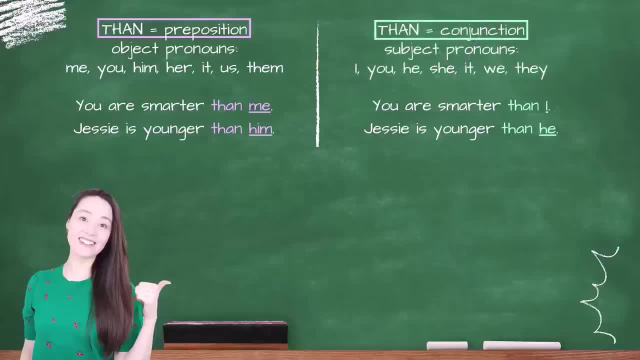 If you consider than a preposition, we use an object, pronoun Me, you, him, her, it, us, them. If you consider than a conjunction, we need a subject, pronoun Ah, you, he, she, it, we, they. 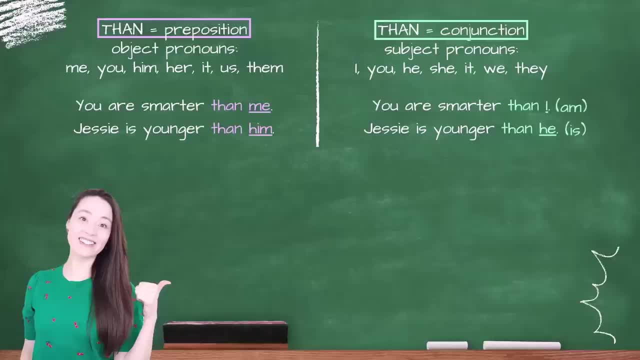 The verb that follows the subject is often given: You are smarter than I am. Jesse is younger than he is. So in these sentences here, it doesn't matter if you use an object pronoun or a subject pronoun. Your sentences mean the same thing. But using an object pronoun is more common and less formal. 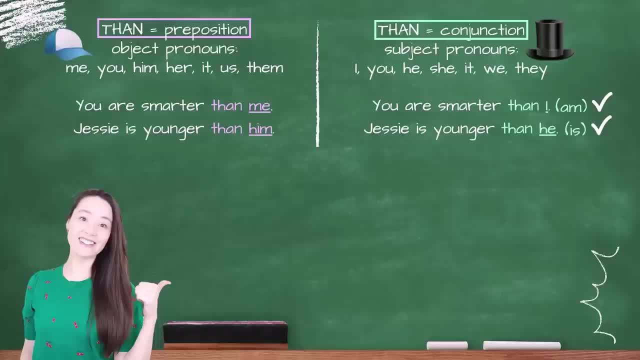 Using a subject pronoun is less common and more formal. To be honest, in my day-to-day life I hardly ever hear anyone using a subject pronoun. So is there no difference between the preposition and the conjunction? Well, let me show an example sentence where using than as a conjunction is better. 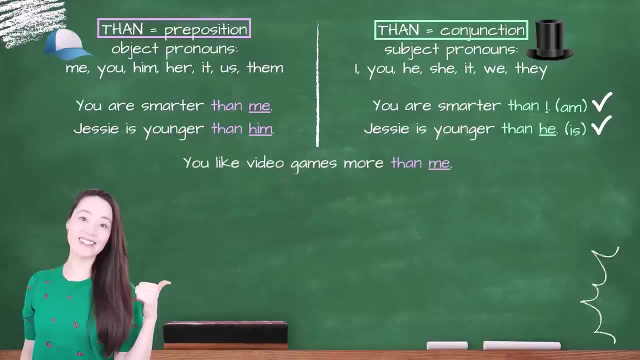 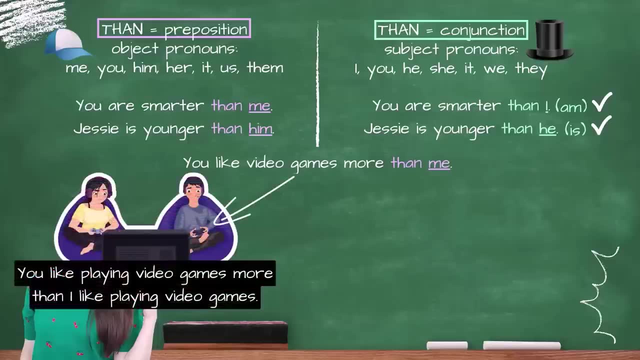 You like video games more than me. This is correct, but it could mean two different things. One, you like playing video games more than I like playing video games, Or you like playing video games more than you like me as a person. 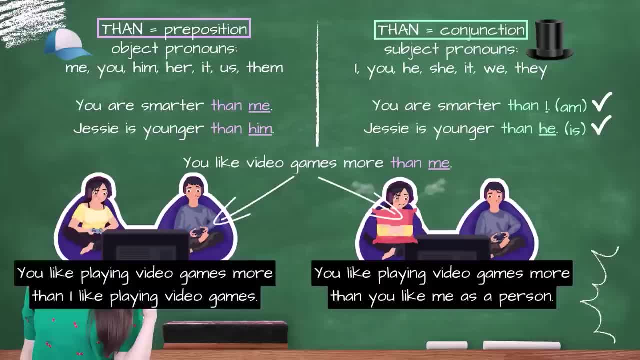 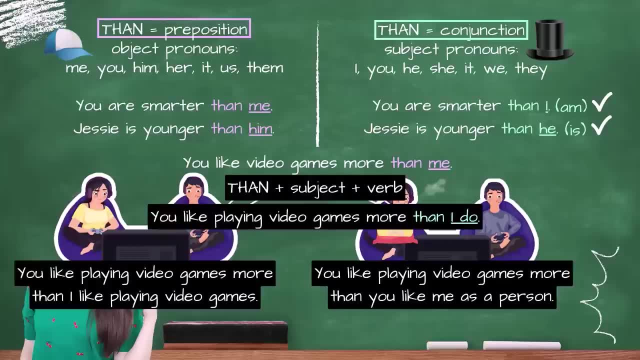 So sometimes, to not cause any confusion, it's better to use than as a conjunction and follow it with a subject and a verb. You like video games more than I do, But normally there isn't any confusion. The context will tell you to keep things simple. 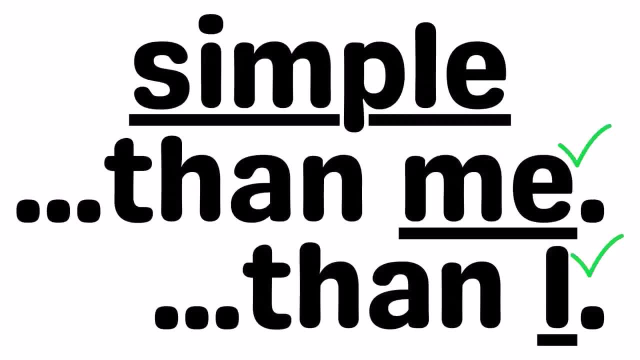 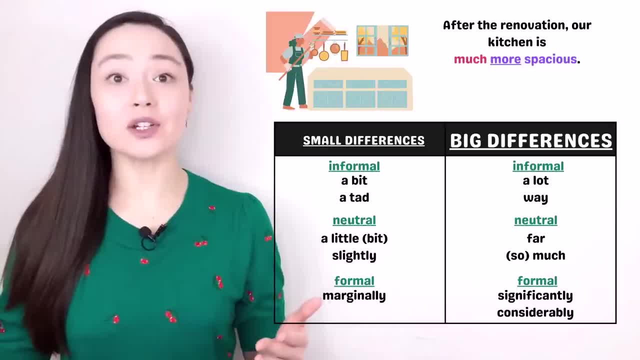 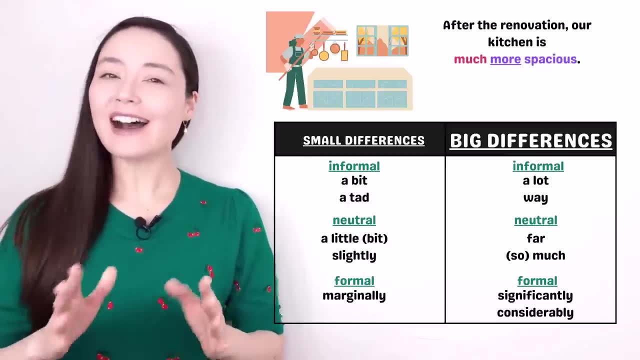 So than me than I are both correct. It's about formality and personal preference. After the renovation, our kitchen is much more spacious, Much more. I know that looks a bit strange, but we can use much to show a big difference. 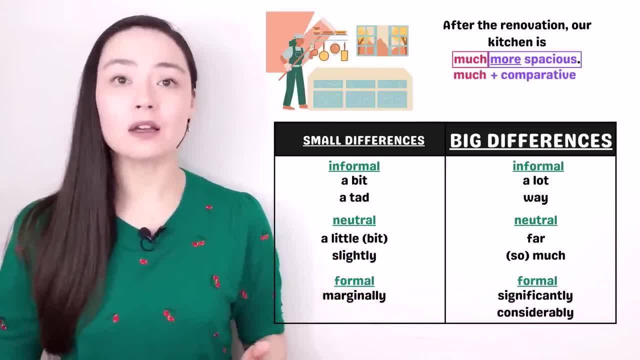 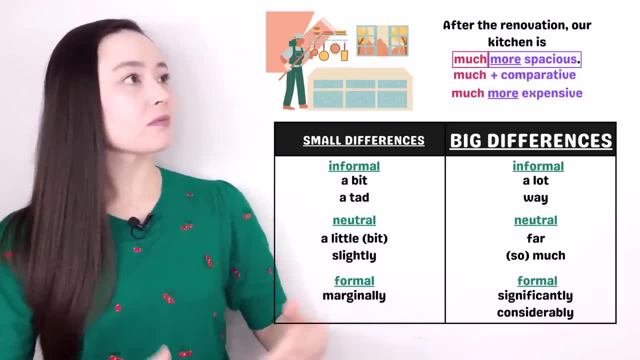 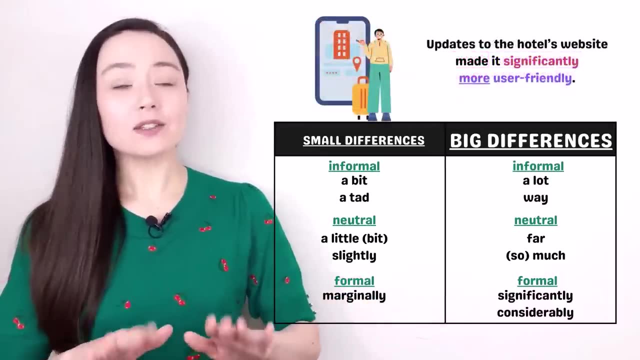 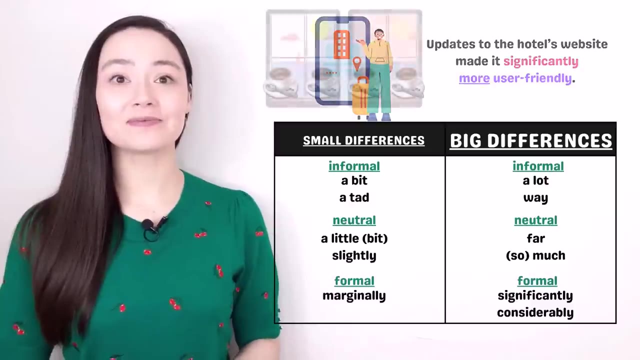 and we can use a comparative. This is really common. Much more spacious, Much more expensive, Much more, Much more interesting. Updates to the hotel's website made it significantly more user-friendly. I used to drink four cups of coffee a day. 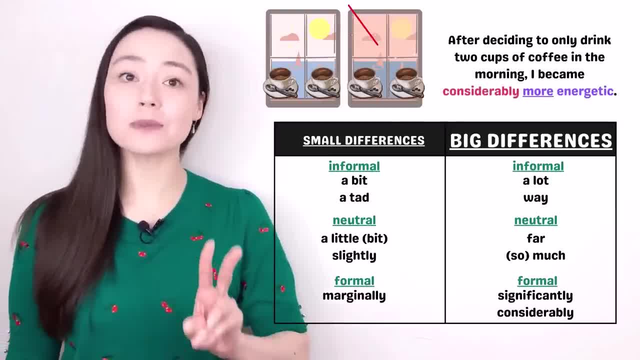 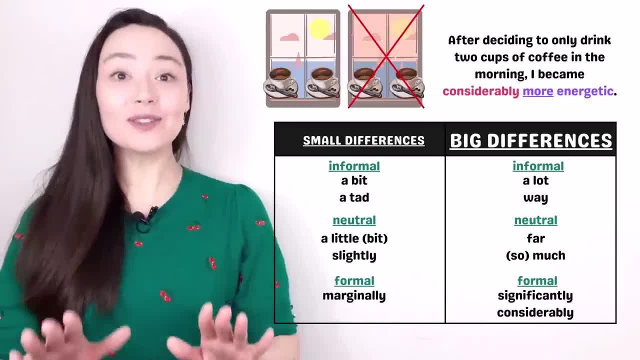 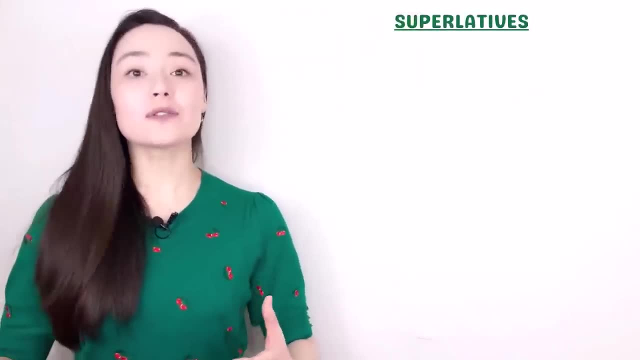 but after deciding to only drink two cups of coffee in the morning, I became considerably more energetic. We've looked at modifying comparatives, but what about superlatives? Well, because superlatives are already the most extreme form, is it possible to show a difference In some ways? 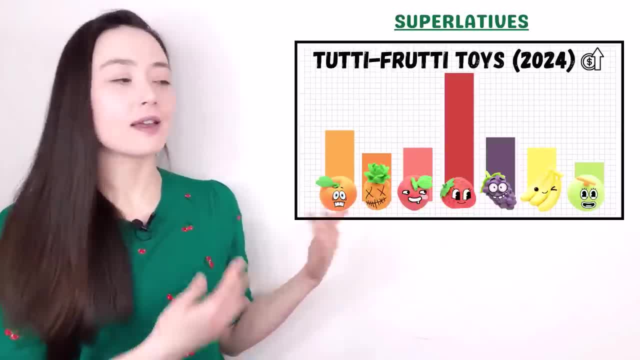 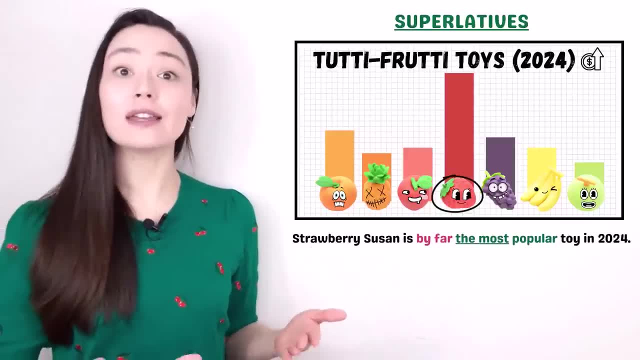 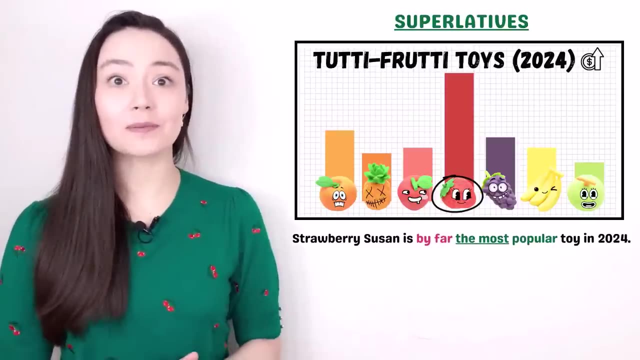 Here are the statistics of a toy company. They sell little fruit toys. Strawberry Susan is by far the most extreme form, At least I think so. By far, By far The most popular toy in 2024.. There's a big difference there. 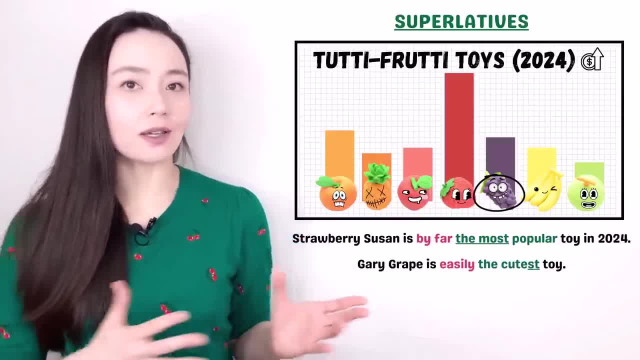 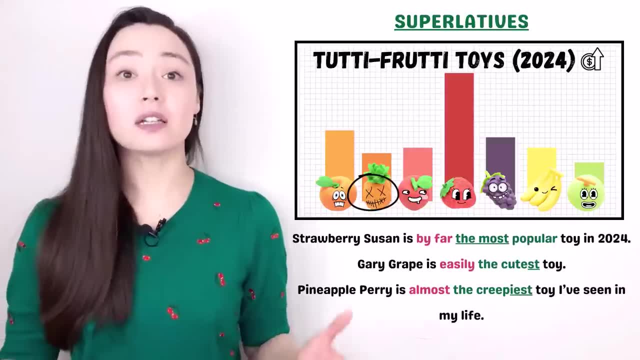 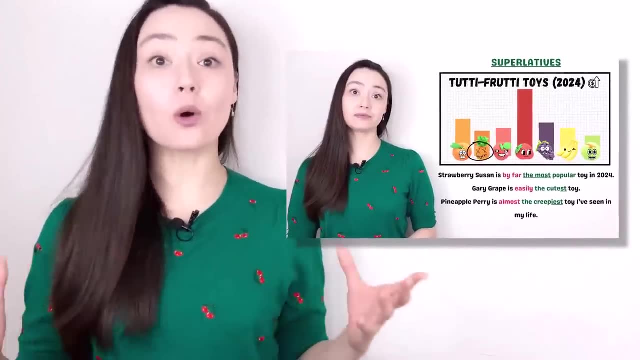 Gary Grape is easily the cutest toy here. Peri Pineapple is almost the creepiest toy I've seen in my life. Let's keep going. Whether we are speaking about small differences or big differences, we're still making the adjectives more intense when we form comparative and superlatives. 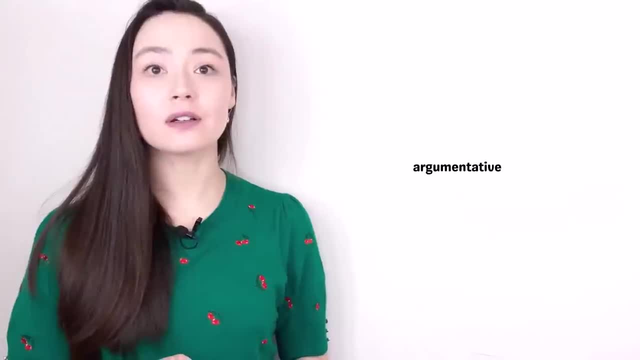 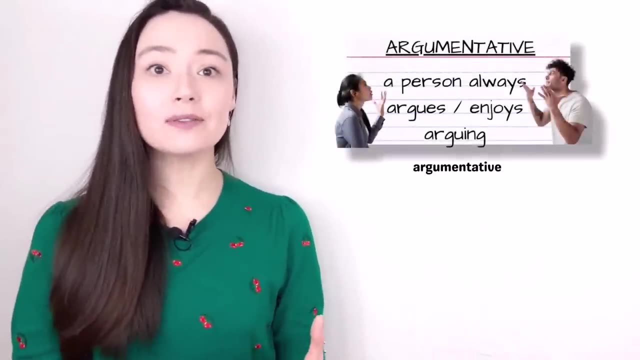 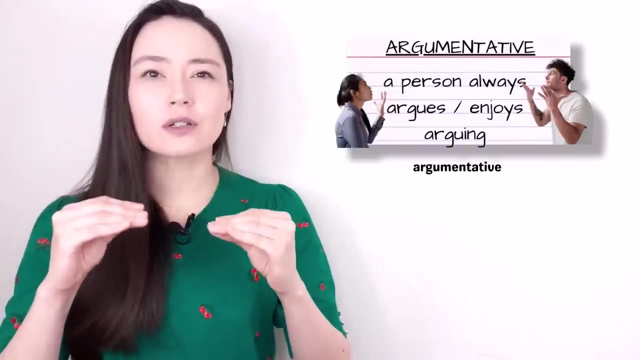 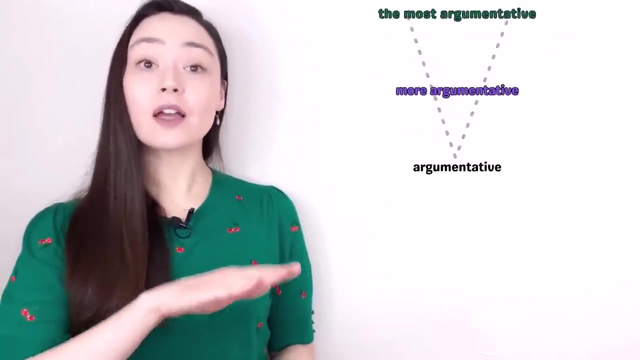 Argumentative- Oh, that's a long adjective: Argumentative, Five syllables. And when someone's argumentative, they like to argue: This is arguing. when you fight with your words, When you say someone is argumentative, that's not a positive description. Argumentative More. 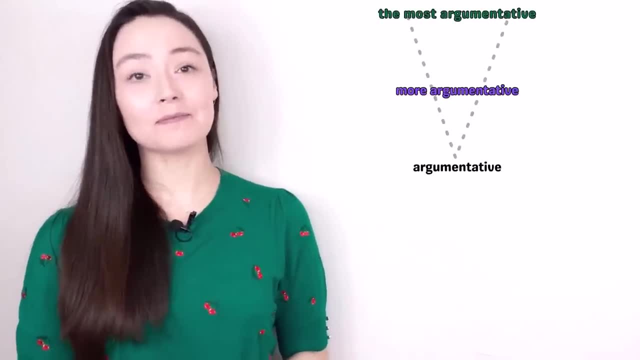 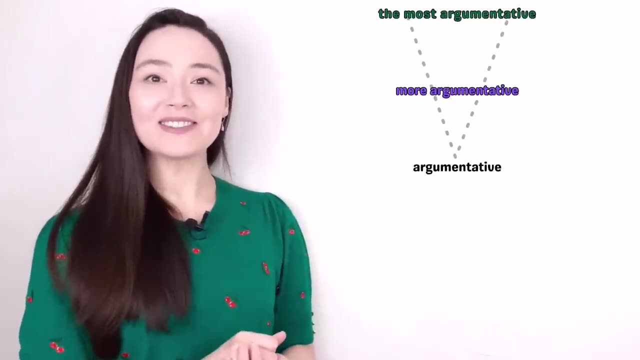 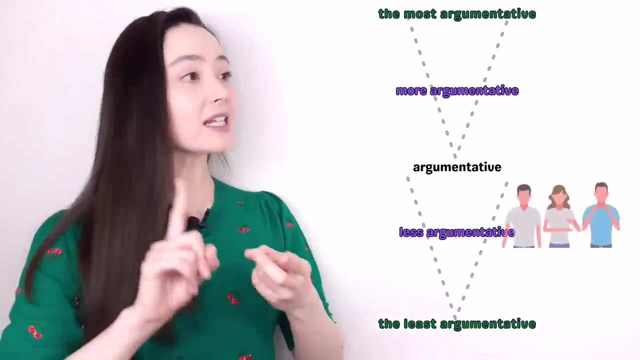 argumentative, The most argumentative. But what happens if I want to make the adjectives weaker, Argumentative, Less argumentative, The least argumentative. Sandy, Paul and Ryan, they're all argumentative people, But I chose argumentative. 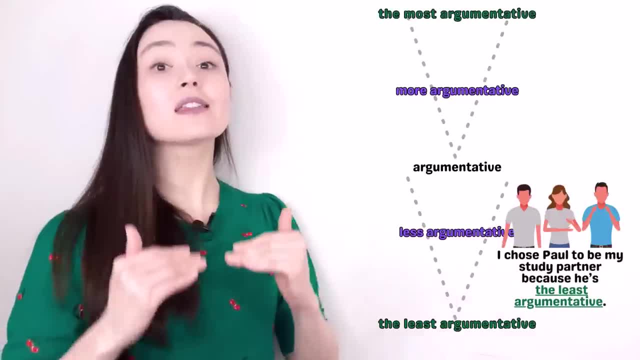 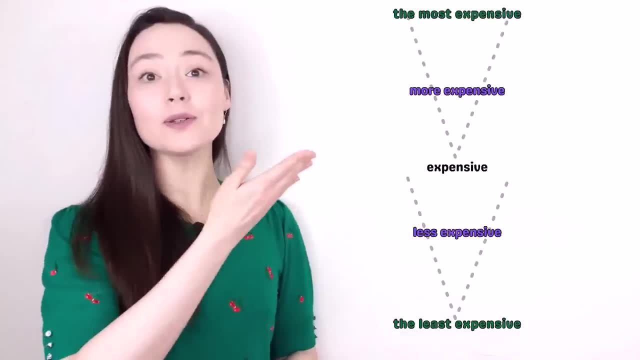 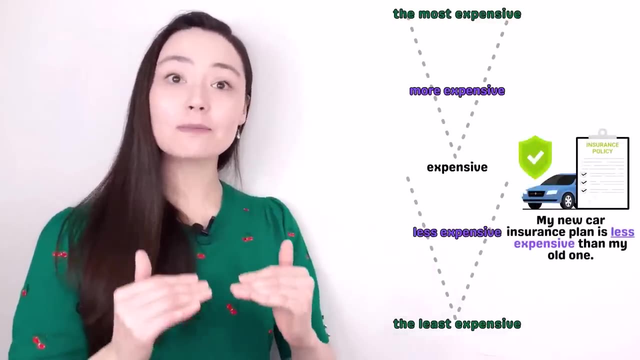 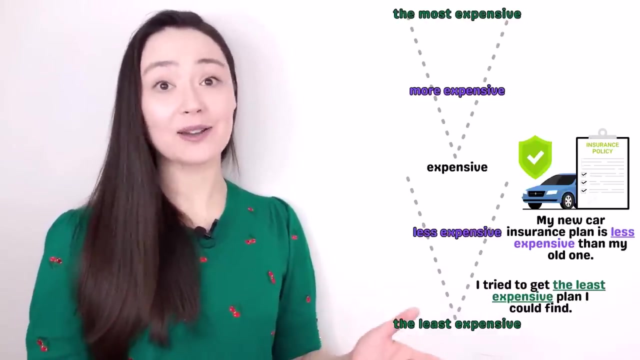 Paul to be my study partner because he is the least argumentative, Expensive. More the most, less the least. My new car insurance plan is less expensive than my old one. In fact I tried to get the least expensive plan I could find. Normally we use less and least. 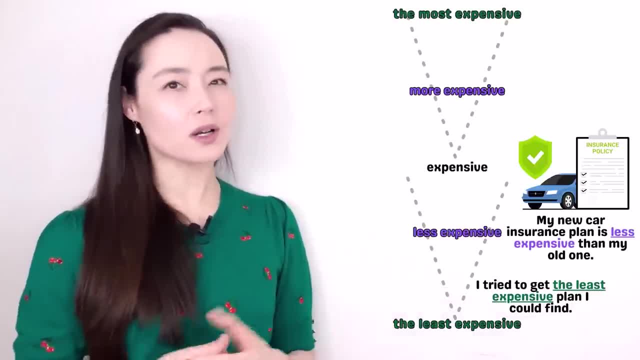 with long sentences, but in this example Paul is the least argumentative. And in fact Paul is the least argumentative And in fact I tried to get the least expensive plan. I could find Normally adjectives, but it's possible with short adjectives. Let me choose hot Friday will. 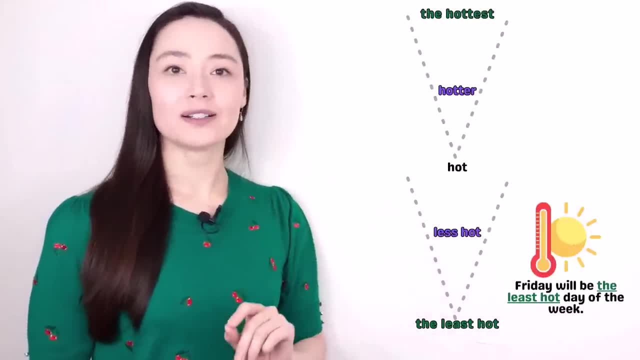 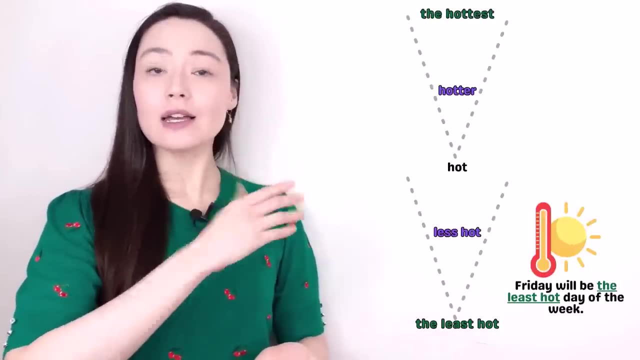 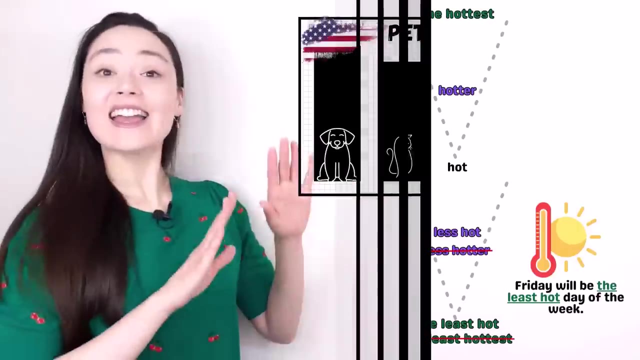 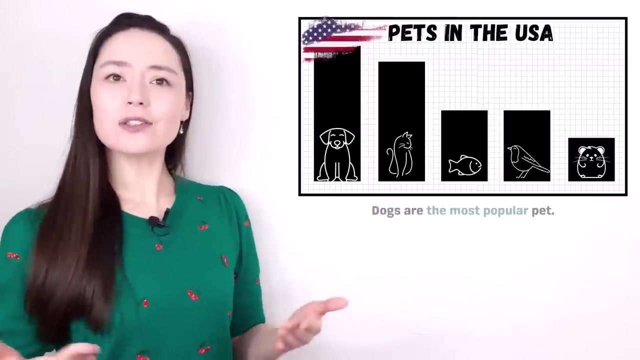 be the least hot day of the week And don't try to form a double comparative or superlative. Hot, hotter, the hottest, But we wouldn't say hot less hotter, the least hottest. Here I have a bar chart of popular pets in the USA. Dogs are the 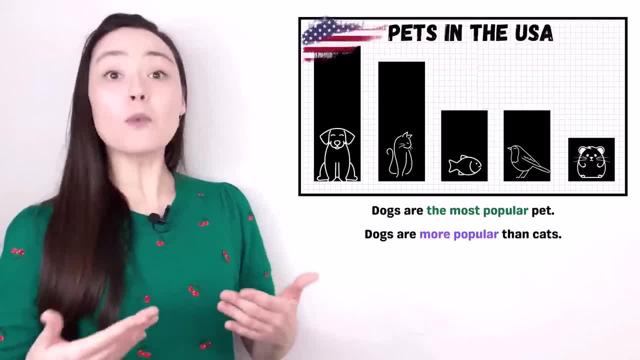 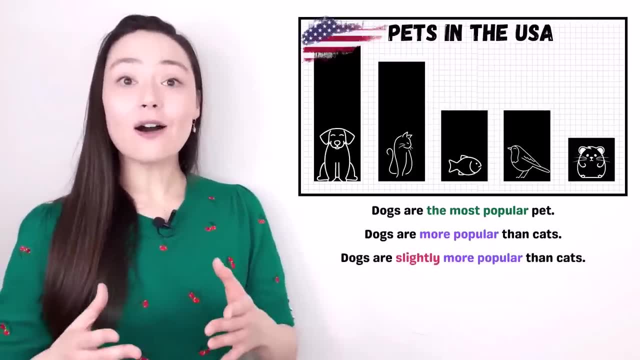 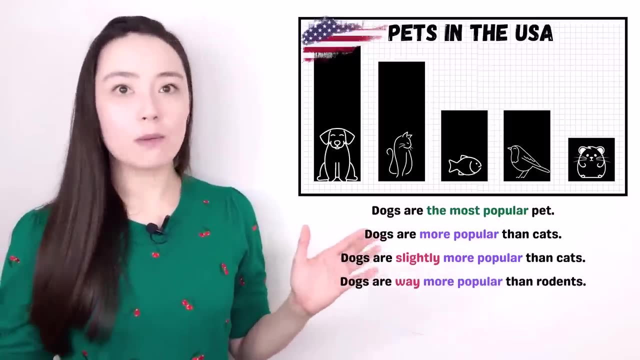 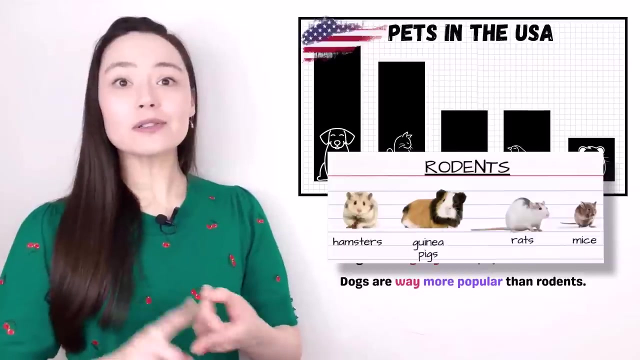 most popular pet. Dogs are more popular than cats, But let's make this more interesting. It's a small difference. I could say dogs are slightly more popular than cats. Dogs are way more popular than rodents. Rodents are animals like this: hamsters, guinea pigs, rats, mice. those are rodents. 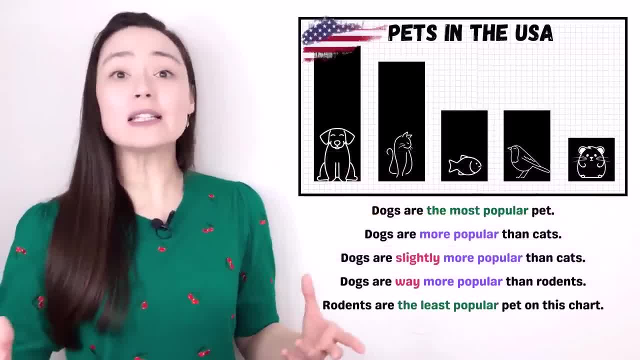 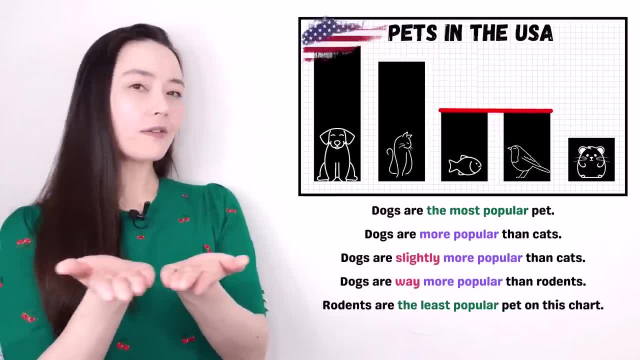 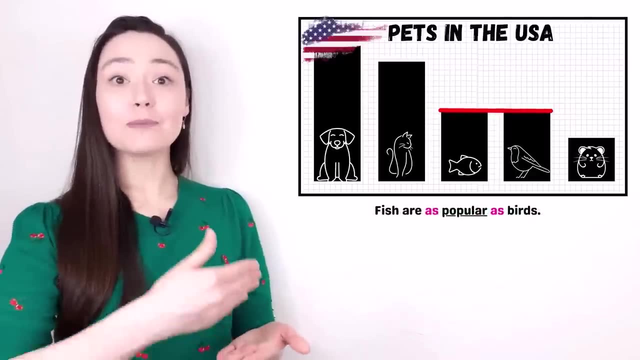 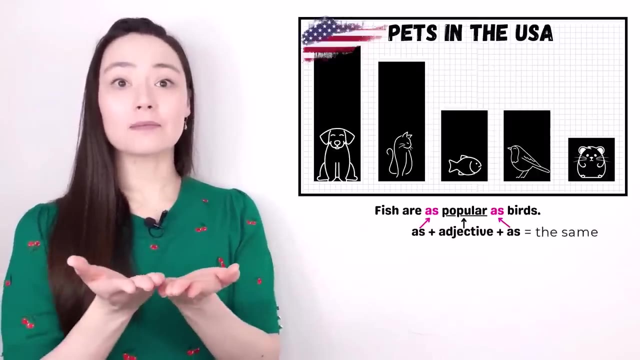 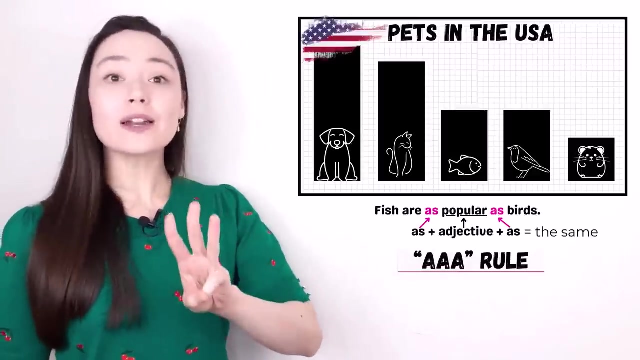 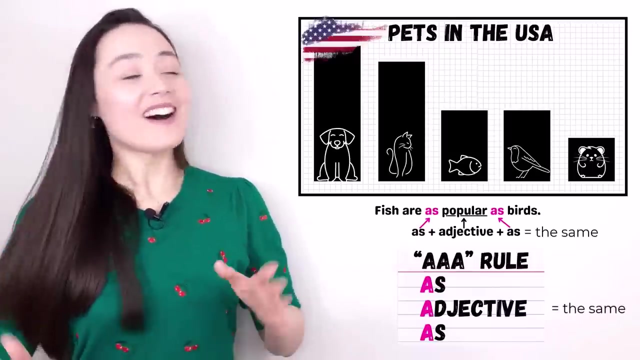 Rodents are the least popular pet on this chart, but fish and birds are the same. What can we say? Fish are as popular as birds. As adjective, as the same. I want you to remember my AAA rule: AAA, three letters, the same As adjective, as that grammar gives you the same. Okay, another chart. 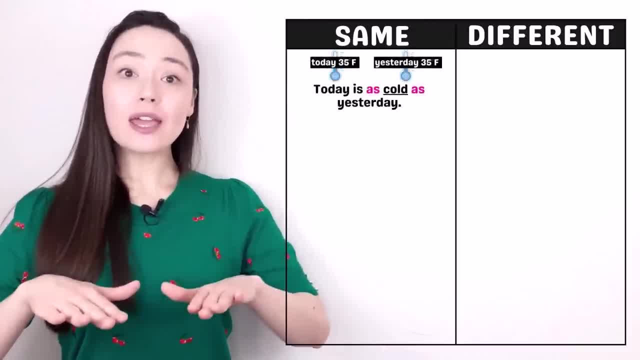 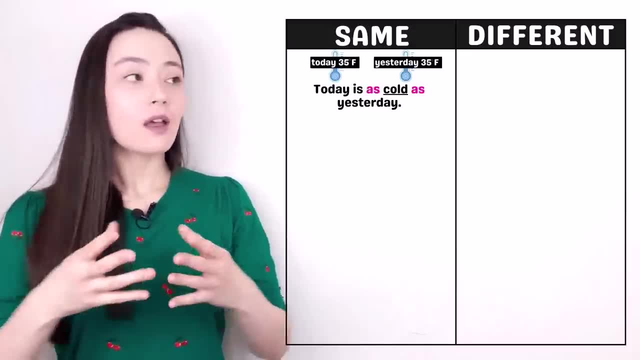 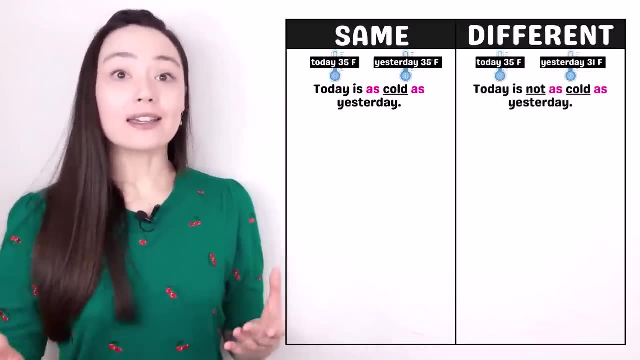 same, different, Okay. another chart, same different, Okay. another chart, same, different. Today is as cold as yesterday. As adjective as the same. Well, I can make this negative: Today is not as cold as yesterday. I can say yesterday. 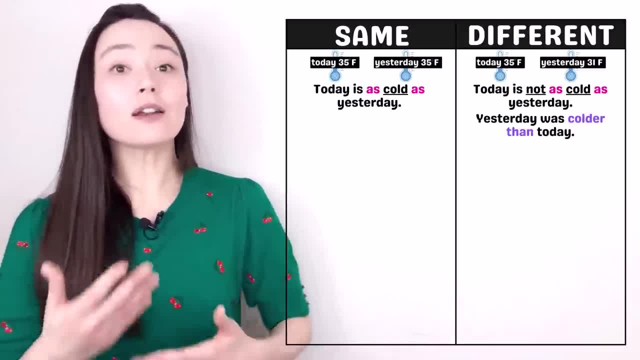 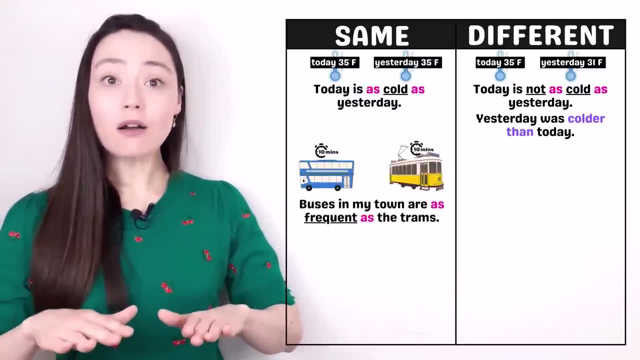 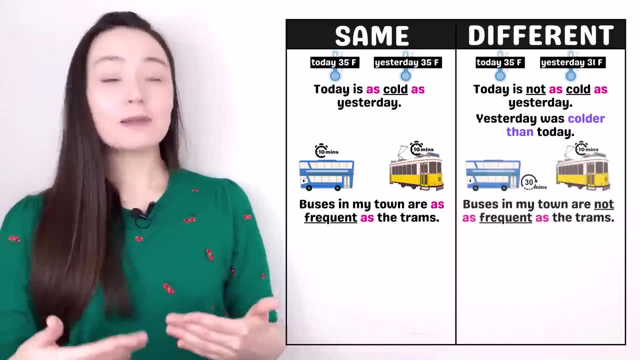 was colder than today. There are a lot of options. It's all about variety. Buses in my town are as frequent as the trams. Buses in my town are not as frequent as the trams. The same Buses in my town are not as frequent as the trams. 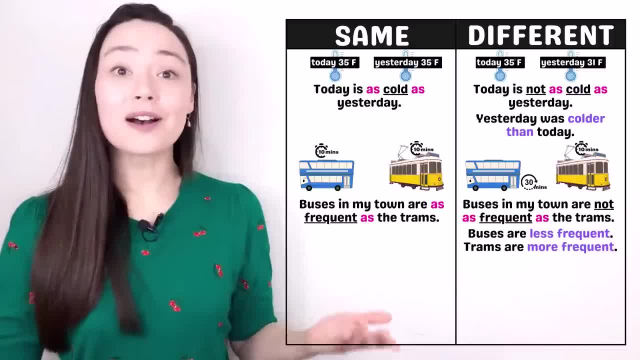 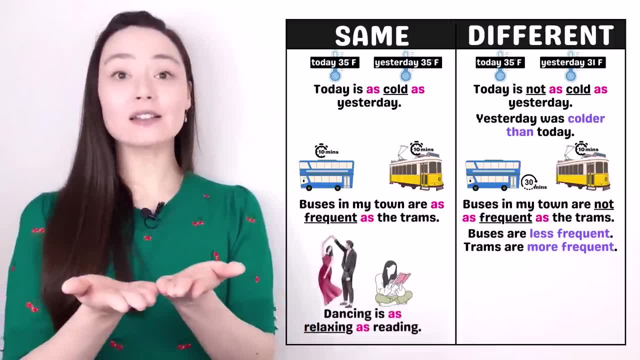 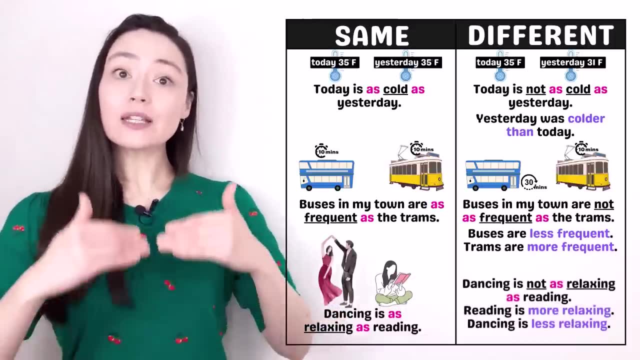 Buses are less frequent, Trams are more frequent. For me, dancing is as relaxing as reading. For me, dancing is not as relaxing as reading. Reading is more relaxing. Dancing is less relaxing, but reading and singing is also relaxing- Dancing is. 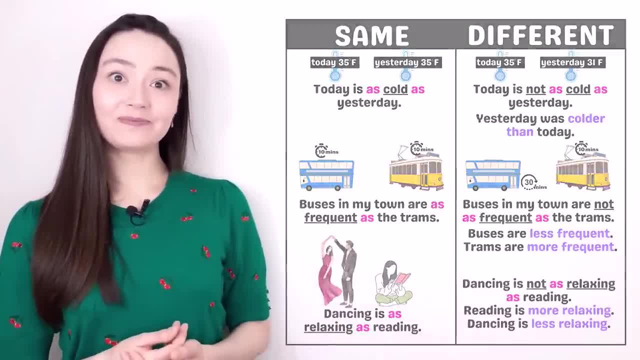 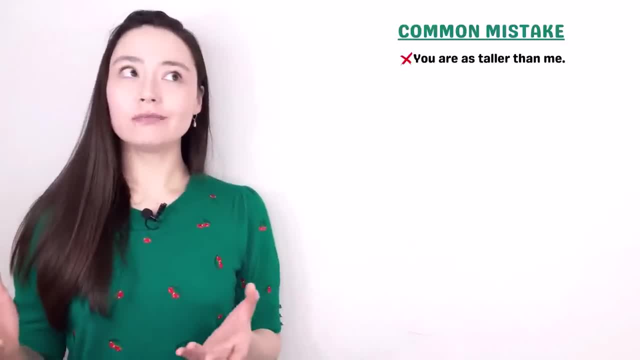 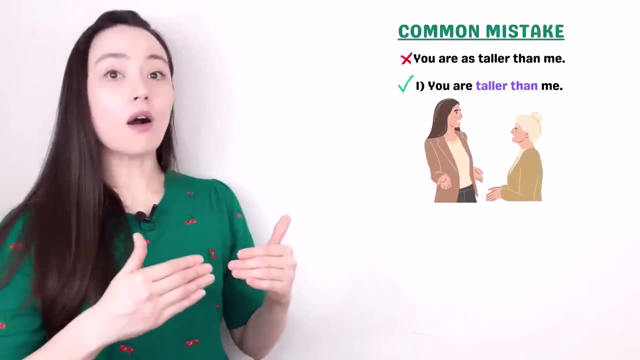 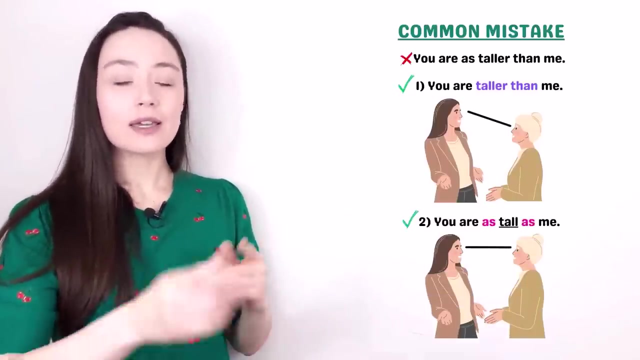 less relaxing. Common mistake: You are as taller than me. We see a little combination here. You don't want to combine the grammar. We can say you are taller than me or you are as tall as me. If you remember the AAA rule, you'll. 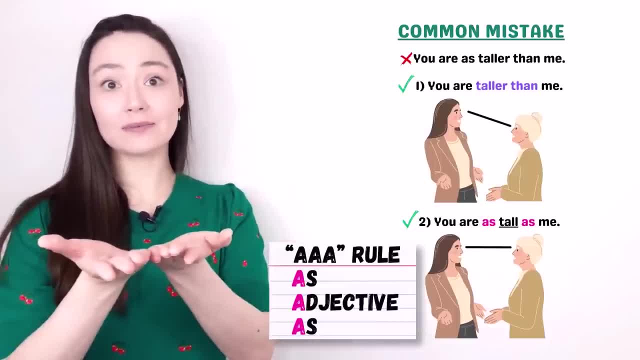 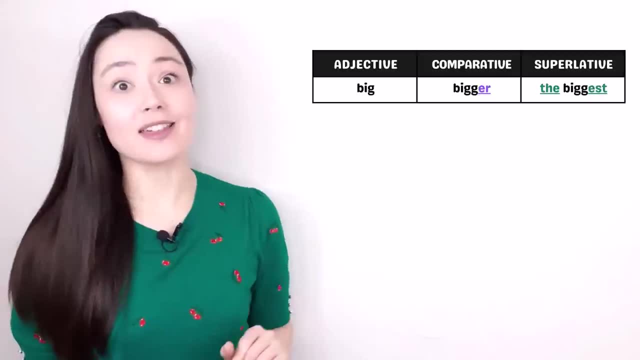 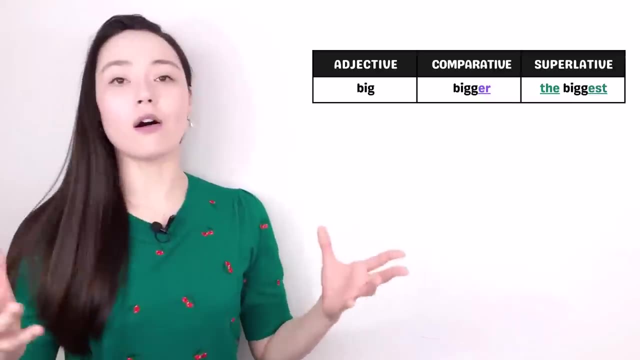 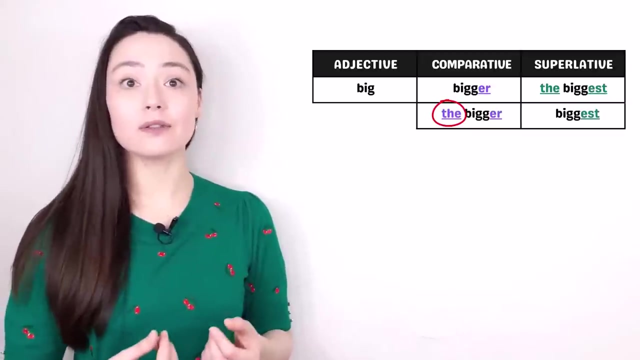 never confuse comparing and similarities. I know there's been a lot of information in today's lesson, but let's look at two more things before the test. You know this: Big, bigger, the biggest. This is what you see on all charts everywhere. But I want to tell you about using the with a comparative and